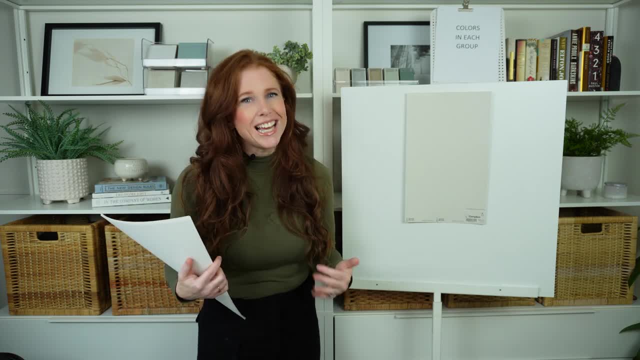 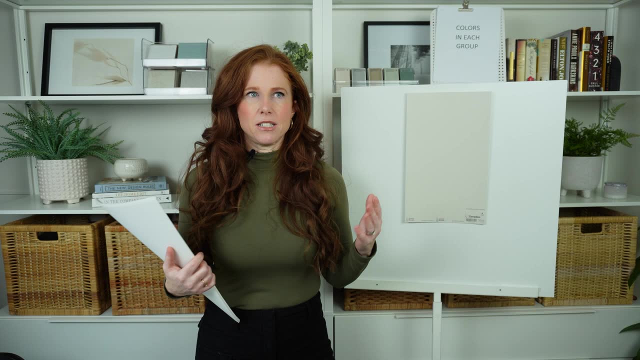 it is so subtle you shouldn't expect it to show up to the party. If it does, it's super subtle. The problem is that if you have finishes like a lot of the homes built in 2010 to 2020 have a lot of grey finishes and people are trying to warm up their spaces a bit, get. 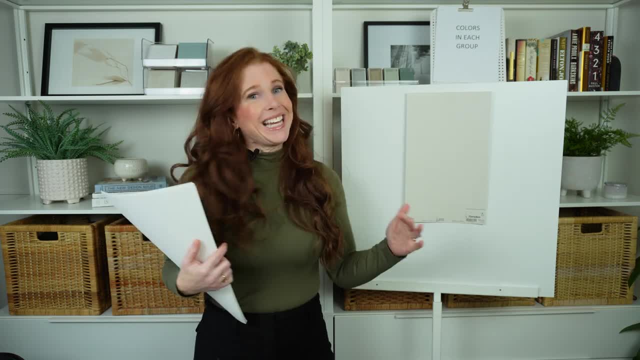 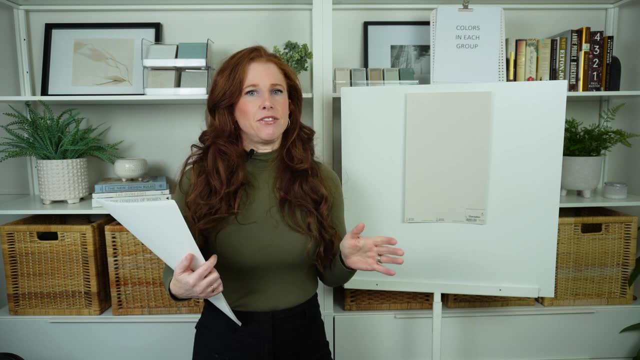 away from that grey on their walls. Agreeable Grey can be a great solution. I'd say 50% of the time it works. The other 50% of the time it's not. The other 50% of the time it doesn't have enough of a violet undertone because those finishes in the 2010 homes. a lot of violet in them, especially like 2015, for reals. So, Agreeable Grey, it's 50-50.. If it works, it's pure magic. If not, I do have a solution that. 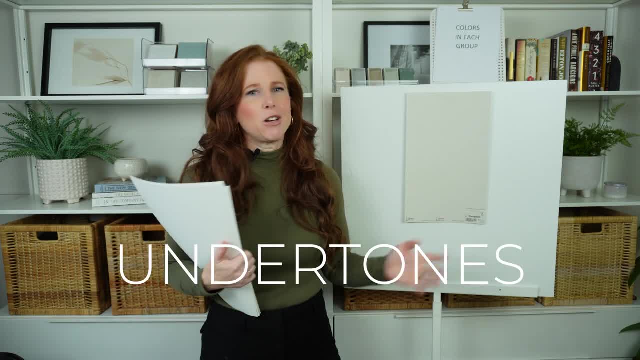 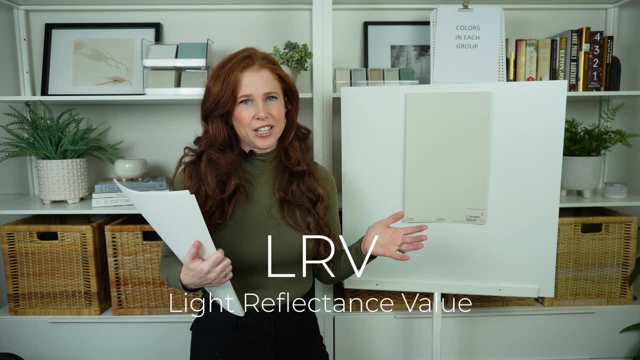 we're going to look at shortly. So long story short undertones, super subtle. Don't expect it to show up. Sample carefully Now. LRV- LRV is light reflectance value. It tells you how light a paint color is on a. 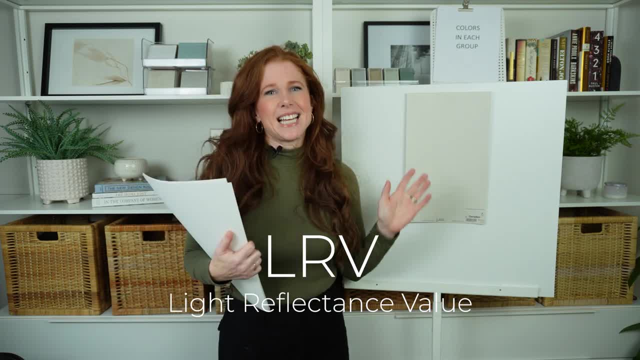 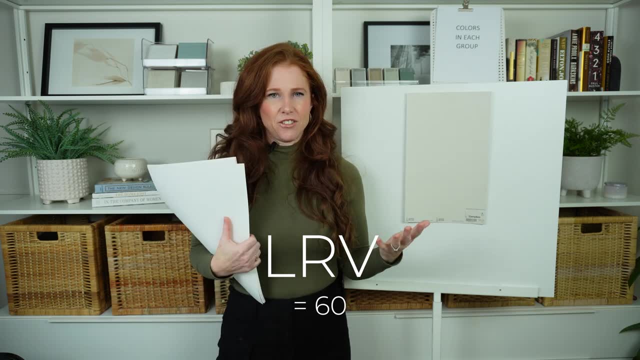 scale of 0 to 100.. Agreeable Grey sits at 60. So at 60, I call this like my happy range between 60 and 70. This range of LRV tends to suit the average room, the average homeowner. 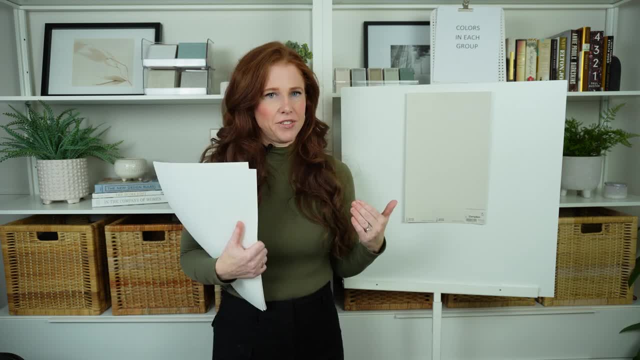 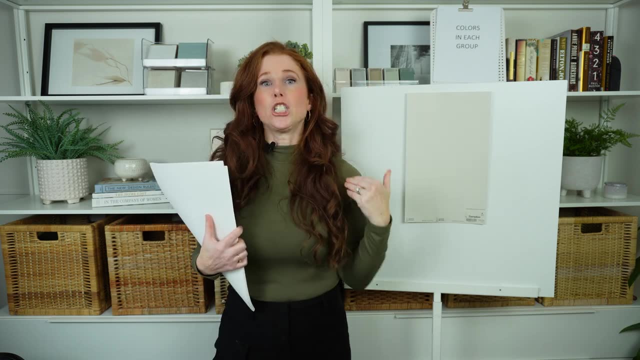 So if you don't know what type of color to look at, find colors with this LRV and I have a great blog post on it. So if you don't know what the heck I'm talking about, read the blog post and it'll be like: so awesome. Now let's say you start with Agreeable Grey. It. 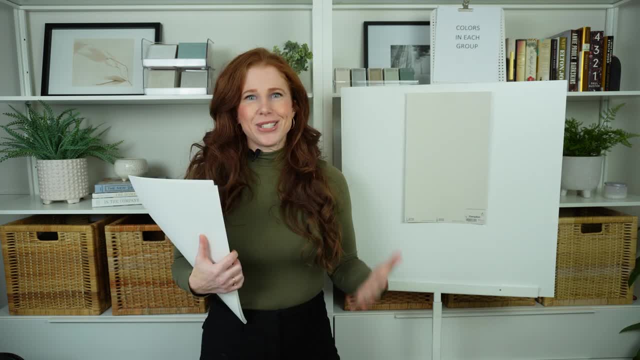 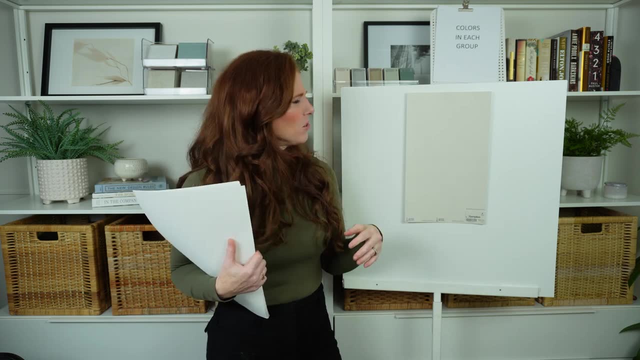 has an LRV of 60.. You'll have some white nearby when you're sampling. because you want to really see the contrast, You might go: oh, that's the perfect depth, I love it. Awesome. You might go: oh, I actually wanted something a little bit darker. Well then, you want to. 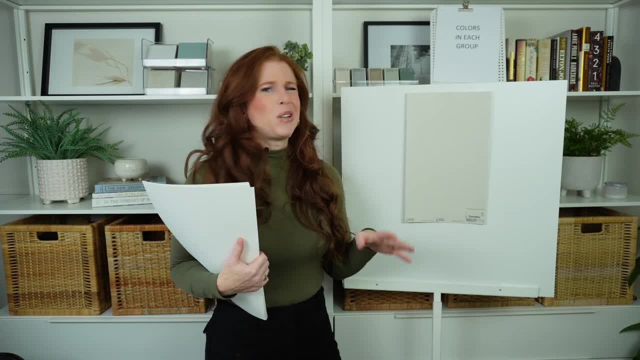 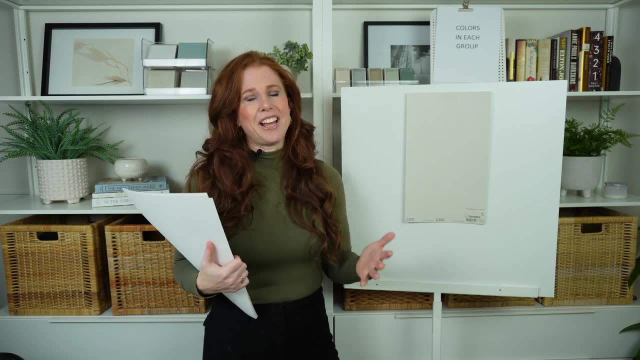 find a paint color with a lower LRV. You might look at it and go, oh, that's a little bit heavier, a little bit more drab than I wanted. You want to color with a higher LRV. Now, how Agreeable Grey looks can vary depending on your interior lighting, the surrounding finishes. 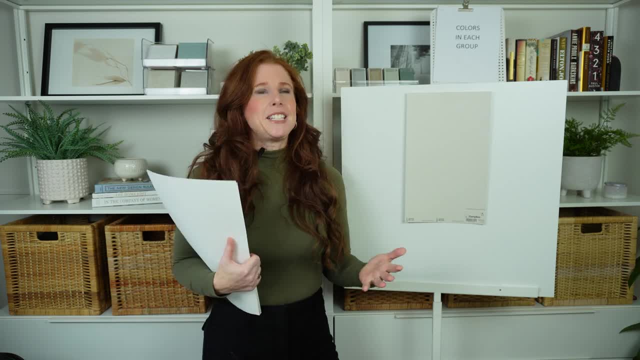 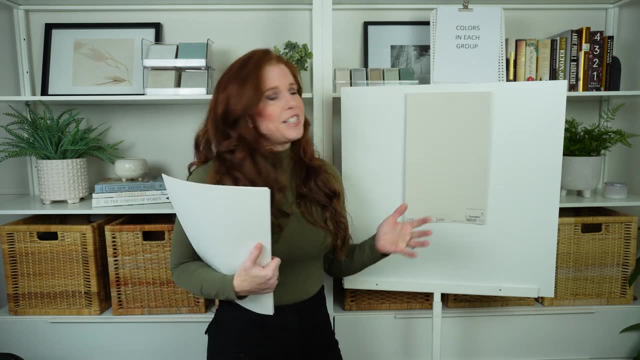 but your exposure actually plays a pretty big part in things. Let's say you have a north facing room. North facing rooms are naturally gray and they can kind of have a bit of a blue tinge to them sometimes. The nice thing about Agreeable Grey is that it still holds. 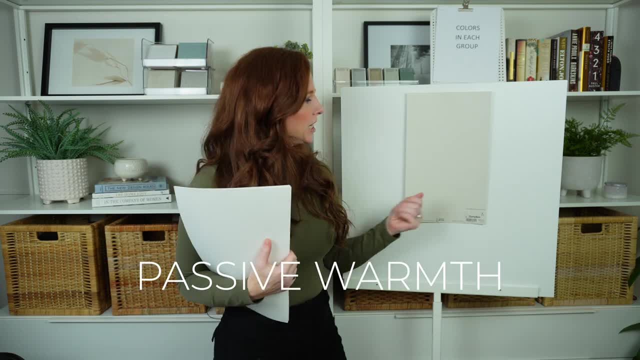 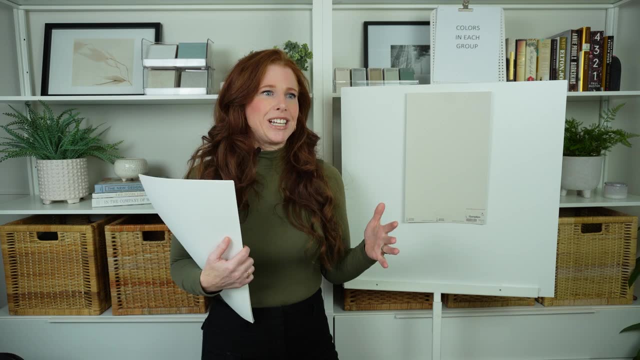 some passive warmth. It will definitely lean that little bit grayer in this light but it doesn't go icy cold like some of the cooler, more traditional grays do. If you have east or west facing light, those are tough, because east is bright, in the morning flat and drab. 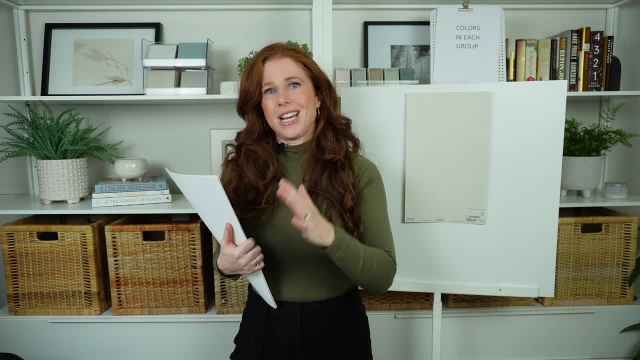 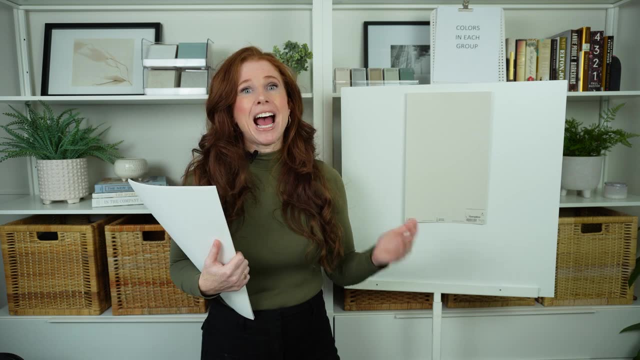 in the afternoon. West is flat and drab in the morning, bright in the afternoon and quite warm as the day progresses. So at that point, well, and with any exposure, it comes down to how much natural light you have, If you have a dark room or one that's not really adequately lit from. 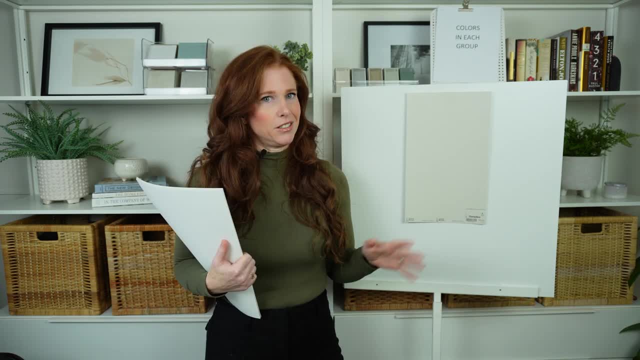 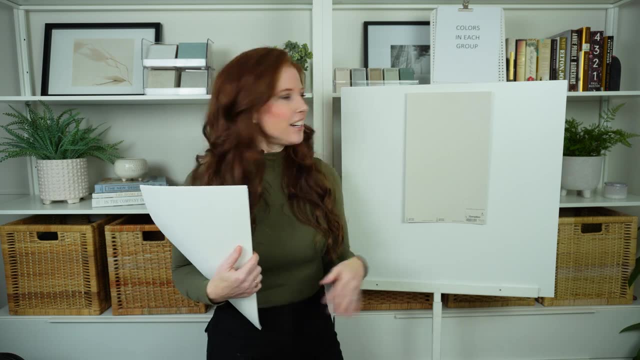 exterior or interior lighting. Agreeable Grey is going to look a little like drab. It's not going to be awesome, a little dingy. If you don't have enough exterior light, amp up your interior light, this kind of color. You know you hit it with like 3000 Kelvins. 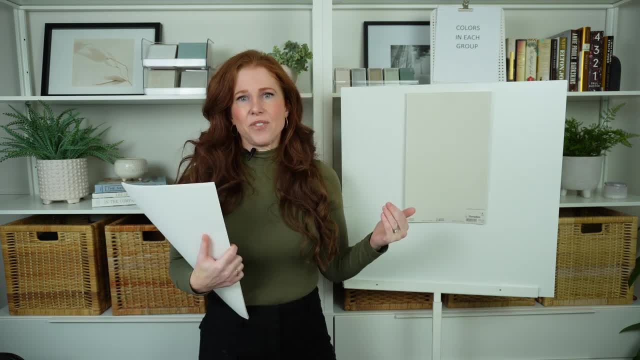 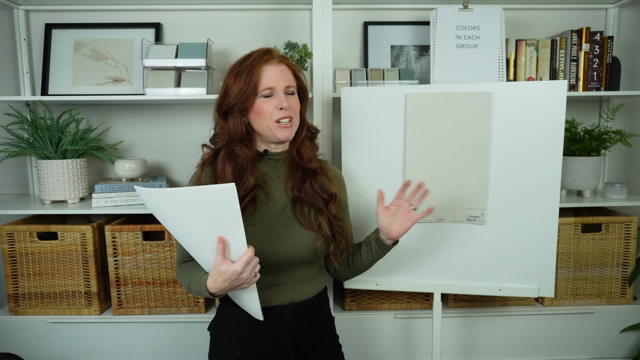 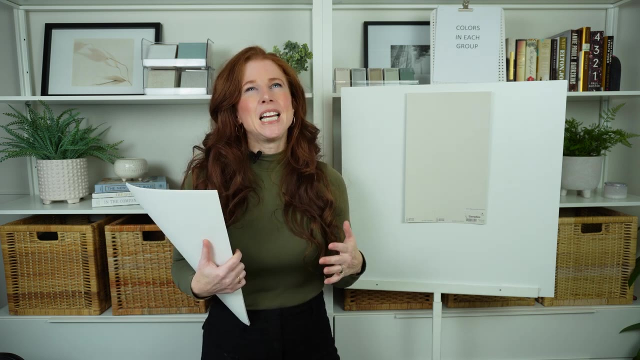 so pretty South facing light. so south facing light or afternoon western sunshine, So lovely, so warm. And a lot of us want to balance that out. but we don't really want a cool paint color necessarily. Agreeable Grey does a great job for that because it adds a slightly cooler 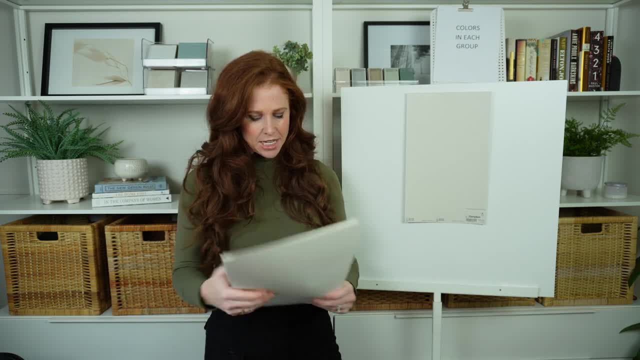 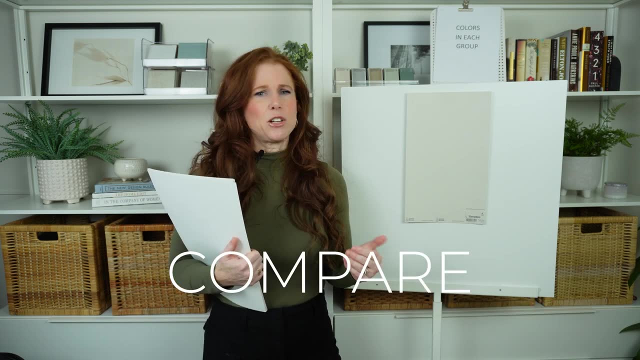 edge without dipping you into the cool tones. Now, when you're looking at a paint color, you never want to pick a paint color based on itself. You need to compare. You might look at one color and be like: that's it, I love it, But if you're looking at a paint, 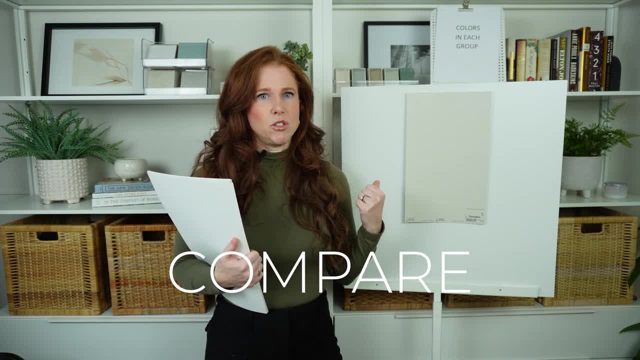 color and you're like: that's it, I love it. Then you might want to pick a paint color and then you compare it to another and go: Oh, I didn't realize that last one had green, purple, blue undertones, or it was actually darker than I wanted. Compare, compare, compare. 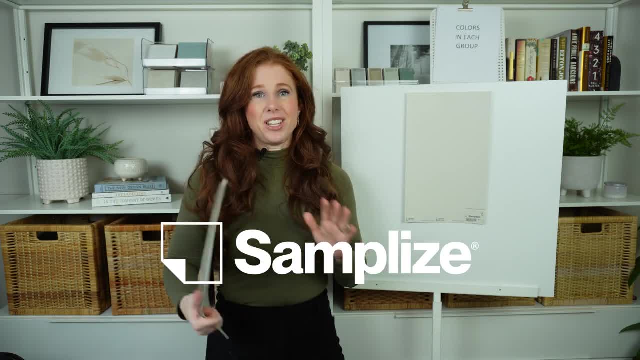 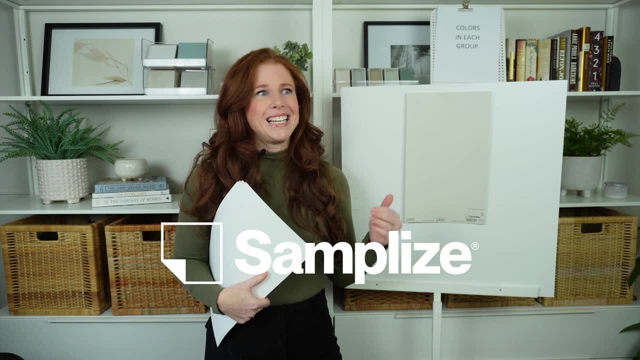 Now I use sample ice, peel and stick because they're made with each brand's actual paint, So they're better than the paint store chips and they're more affordable than your messy sample pots. and they deliver to your door the next day, So no brainer for me. Now. first, 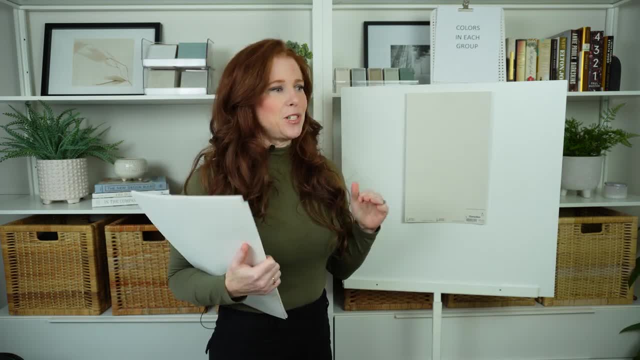 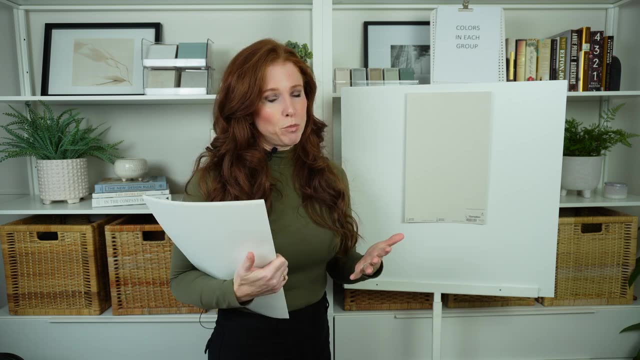 comparable. Oh, by the way, my next video, Unagreeable Grey, is going to be colors that look good, with agreeable gray, as well as a few countertops and fun stuff. This is just about looking at other options to explore that are similar to a little bit different. 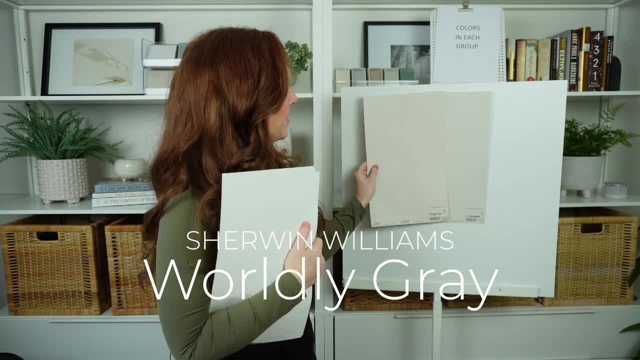 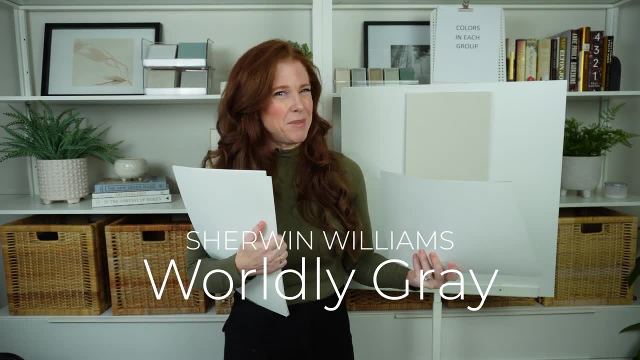 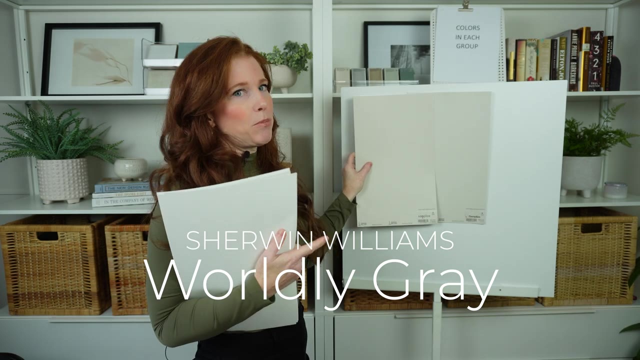 than agreeable gray Sherwin-Williams, worldly gray. So as you can see here, worldly gray, little bit more depth. So I'd say maybe I could be wrong, Maybe it's like 58 or something in its LRV It's also it's had a little bit more of a muddy look and of the two is a bit. 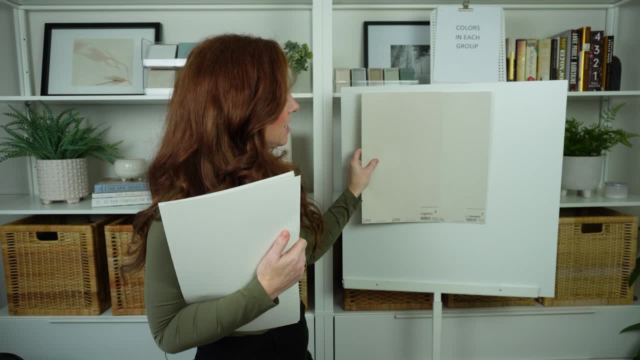 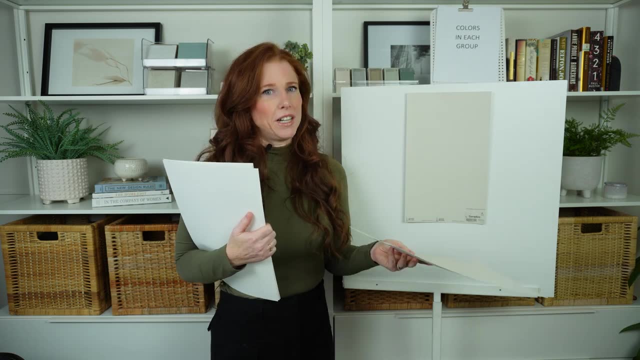 more likely to grab that little flash of green. When I do my online color consulting, I never recommend worldly gray, or if I do, it's like one in a hundred times. So if you're looking at these two agreeable, gray is probably the. 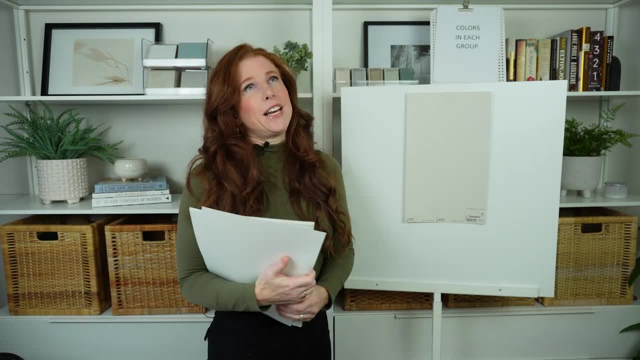 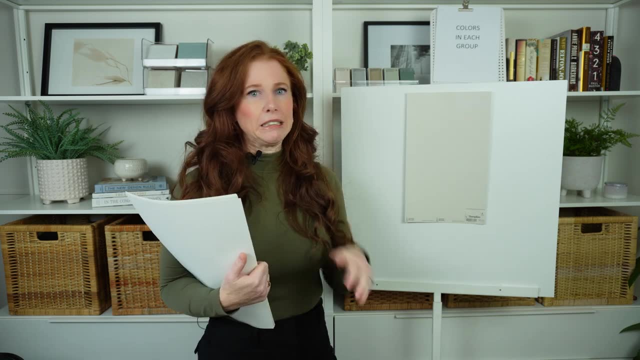 better color for your home. It tends to work more often. Now, sometimes people are like, Oh, I want a lighter version. According to Sherwin-Williams, the off-white version of this is incredible white, Don't do it? Uh, incredible white can be very pretty If you. 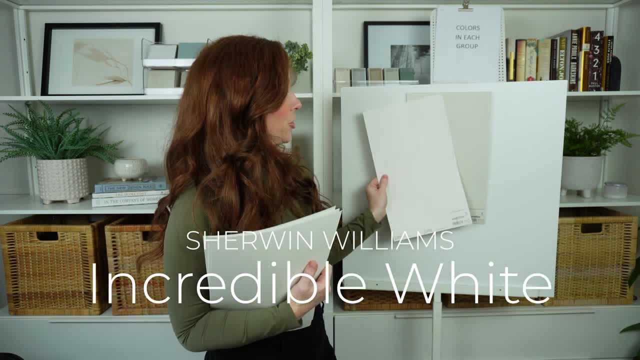 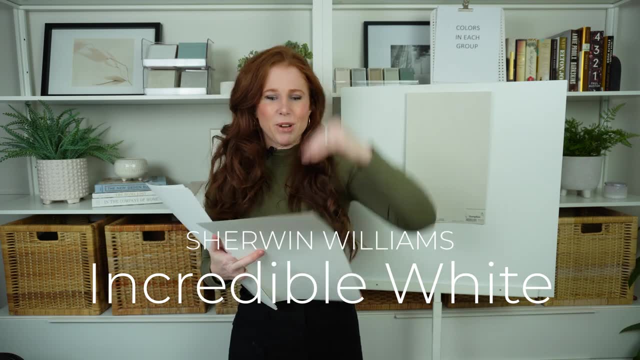 like a purple and pink undertones. this is going to be your jam, Right? So that's the deceiving part. is you look on these strips and you say, Oh, there's the off-white, there's the dark. They all relate, They all look good. They don't always. 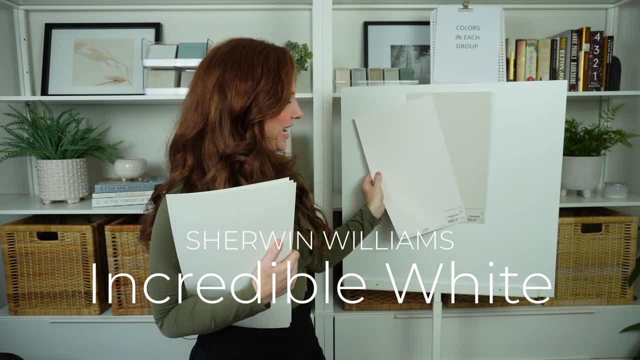 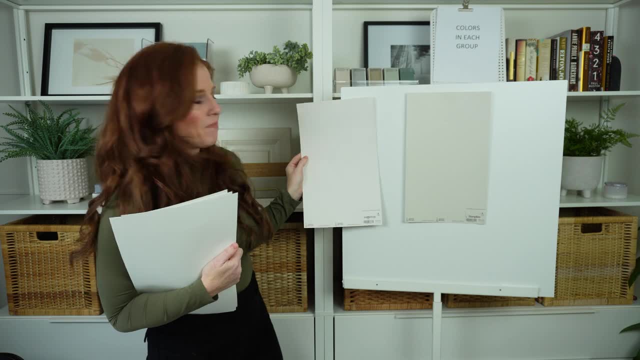 look good And, case in point, incredible white. That's a hard no on that. Again, you might look at this all on its own and be like: Oh, that's pretty, I love it. All of a sudden you put it with white. you go: Oh my goodness, There's some pink in there. Sherwin-Williams. 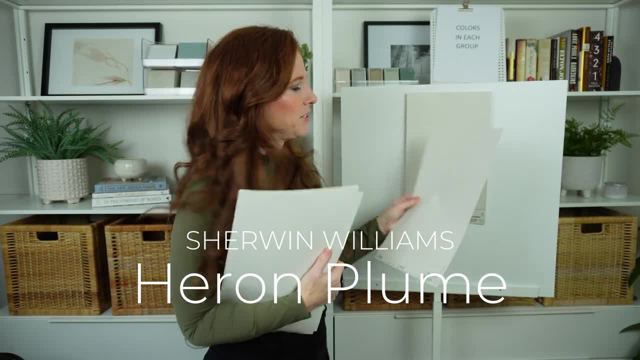 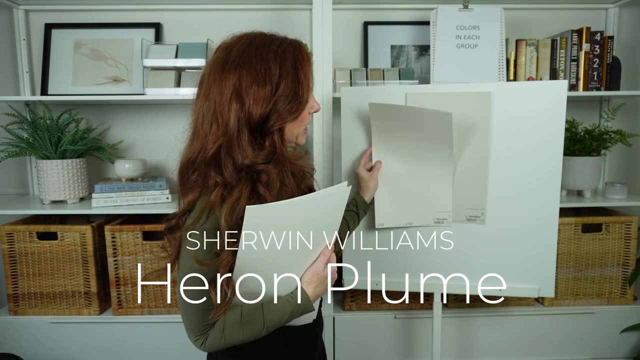 hair and plume. Let's see, Sometimes I just grab these without thinking. I just kind of like go, Oh, catches me. Um, that's a little bit better version of an off-white, even though it's still pretty pink for agreeable gray. Agreeable gray is a tough one. Actually, I'm 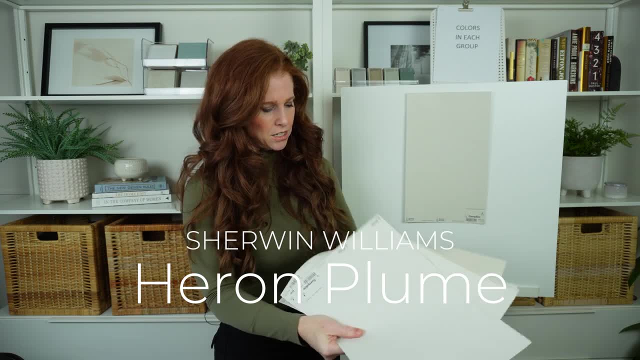 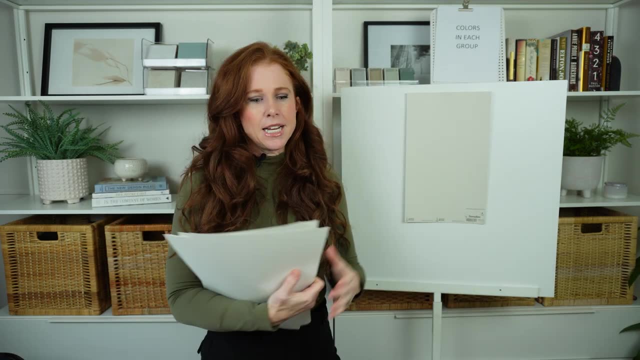 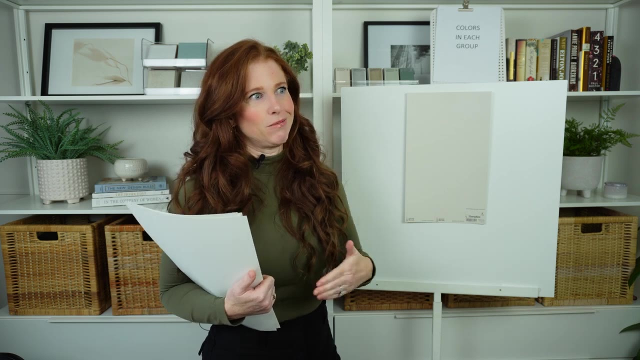 going to grab. where is a new gray? I knew, I knew There we go. So right now, agreeable gray is pretty hot for cabinets. The thing is, as a cabinet color, this depth is really tough. It makes it tricky to pick a wall color. If you don't like white, Um, in which case. 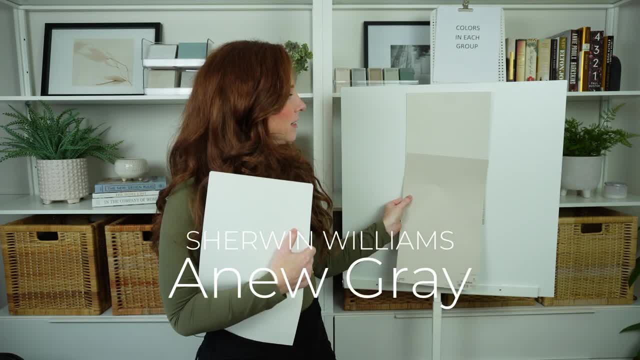 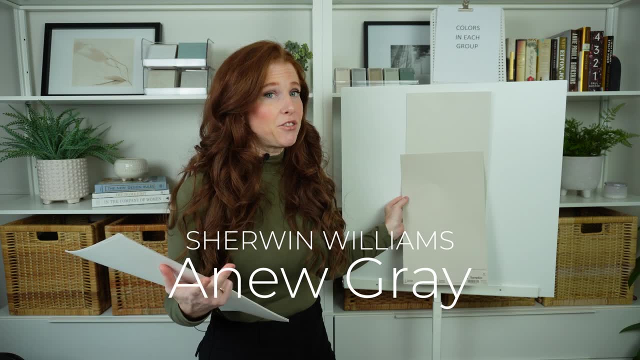 sometimes I say: well, let's bump things down a bit, In which case we look at a new gray. It really picks up what agreeable gray is throwing down. It just adds more depth, gives you more versatility for wall colors. Now, if you're not painting your cabinets and you're 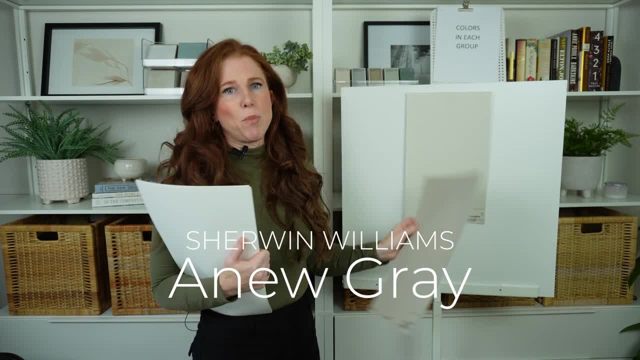 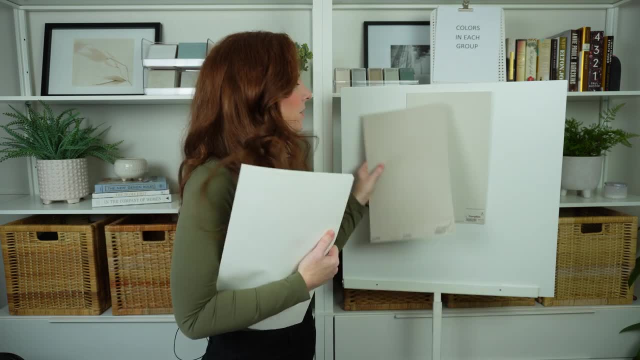 looking for your walls. of the two agreeable, gray is way more popular again because of its LRV. I don't know what this guy's at. I could make it up and say like 53. I don't know, But generally for the average room this is too dark, Unless you want to add some. 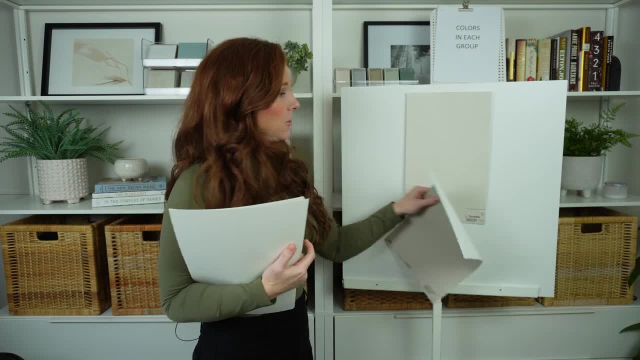 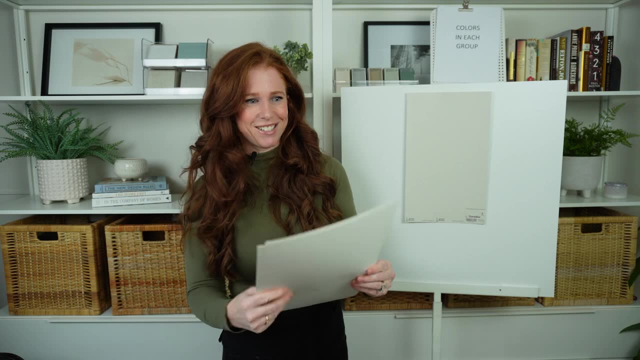 visual weight. If your room is super bright, blown up with light, agreeable gray will wash out. You might really like a new gray. Am I talking too much? I know I talk a lot. I get very excited about this stuff. Sherwin Williams City Loft- Again another off white. 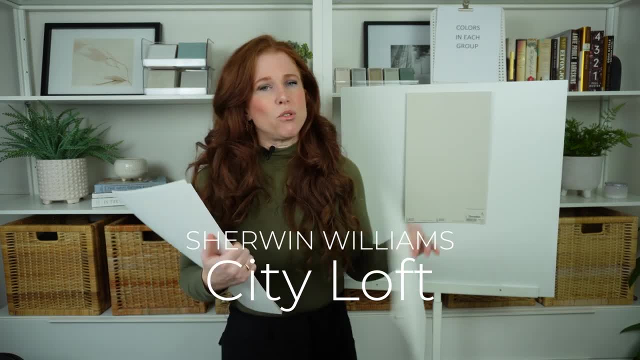 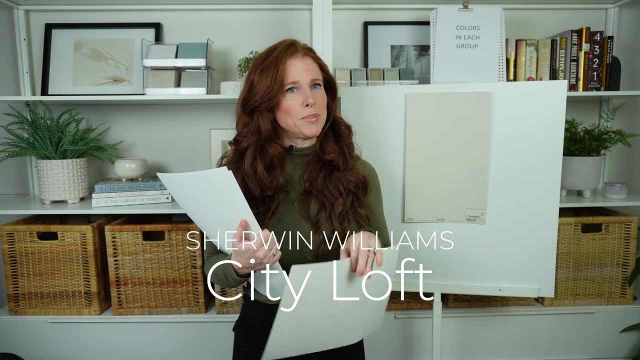 That's gorgeous. I love it. The thing is, if agreeable gray had a little bit of a violet undertone, it would love these. So this is showing you how sneaky that green is, how it stops agreeable gray from going violet without being green. 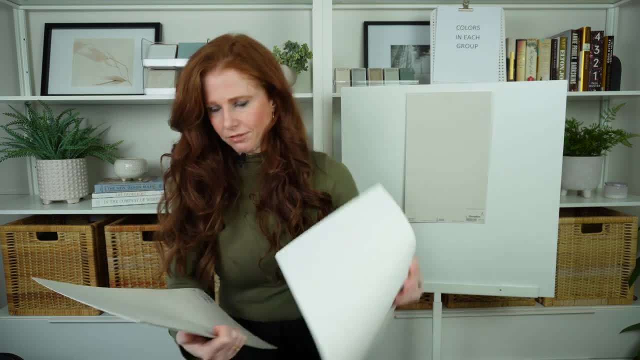 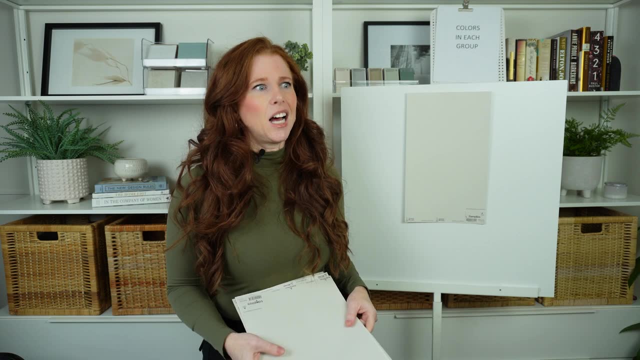 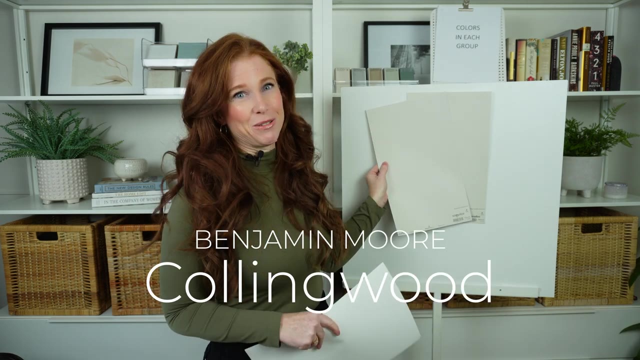 So there you go. Case in point: Ah, Benjamin Moore, Collingwood. So you look at agreeable gray. you love the general look of it, but you're like I think it looks a little green in my room or it's not quite grabbing the violet undertone. I need it to Enter Collingwood. 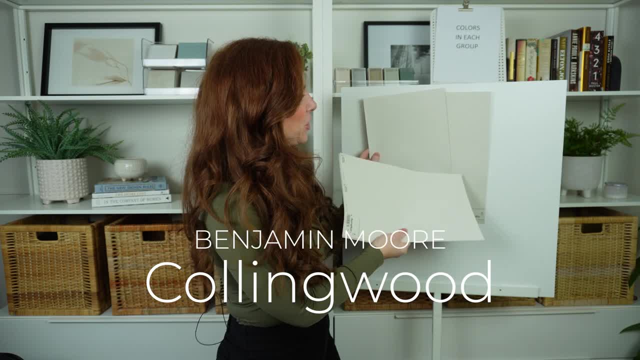 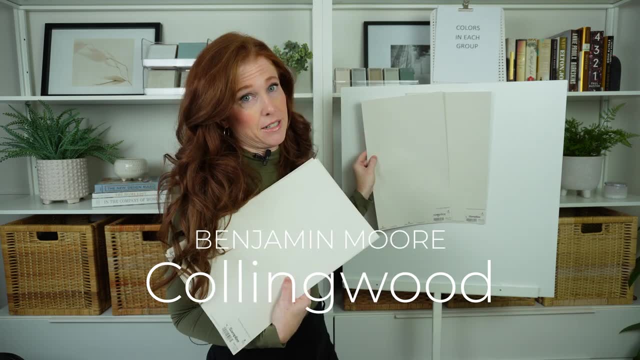 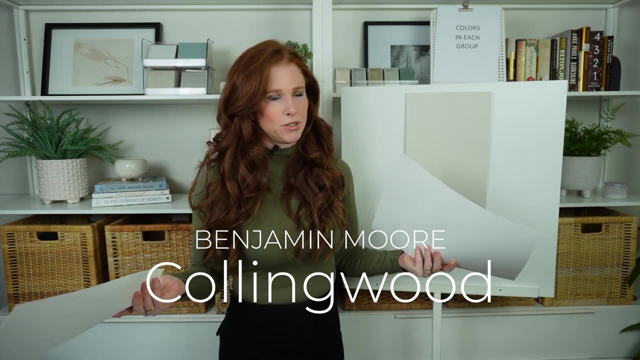 Do you see it Seriously? So there's Collingwood. Do you see that little tiny bit of like almost muddy green in comparison? I hope you do, Cause this is really exciting to me. So Benjamin Moore, Collingwood tweaks that now And again I have- I have blog posts on all of these. 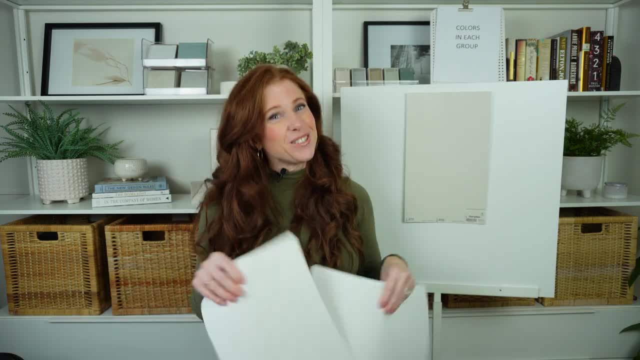 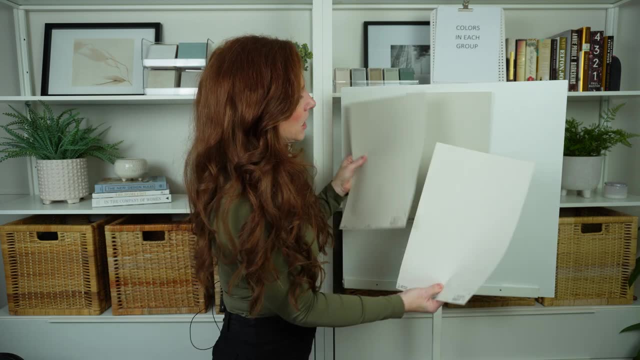 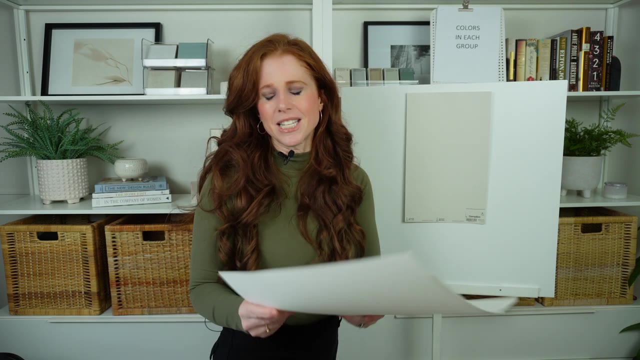 on Kylie. Emma chairs, I have videos and I'm updating all my videos So they're even more awesome. Uh, so look at the difference. There's City Loft with agreeable gray. It's like wah-wah, We put it with Collingwood, Oh, like everything's happy right. So undertones, undertones, undertones. 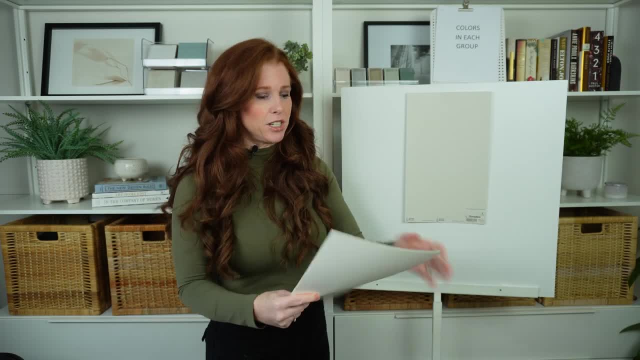 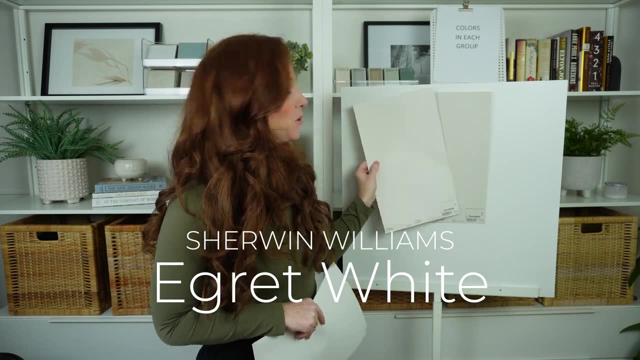 And the only way you can know is to compare and what you think suits your home. Your home might disagree with you. Sherwin-Williams, Egret, white- Again, passable If you were putting these in rooms adjoining each other. great, Like you know. bedroom, bathroom. 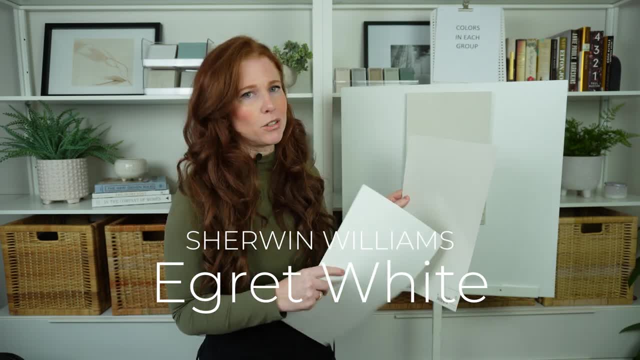 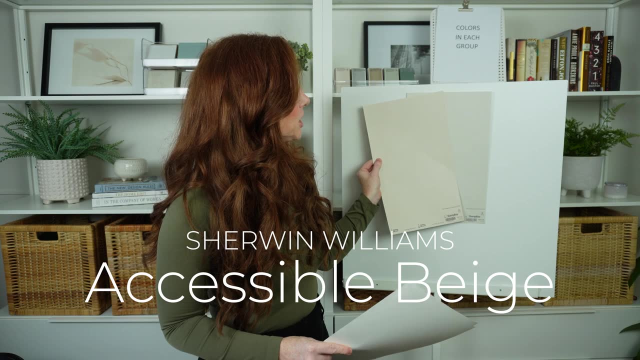 no problem. But you know, cabinet, wall or wall cabinet, Nope, Agreeable gray is a tough cabinet color, Beautiful wall color: Accessible beige. When I do my online consulting, in the questionnaire I ask all these questions. So one of them is like: are there any colors? 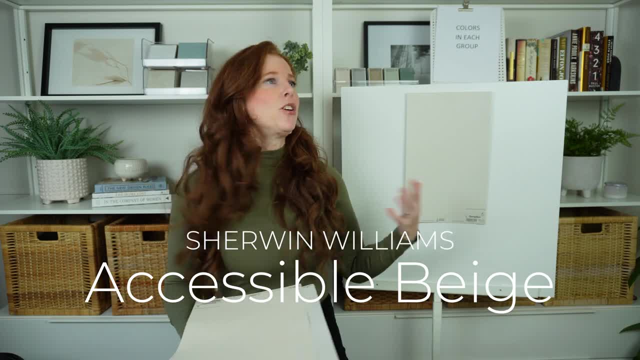 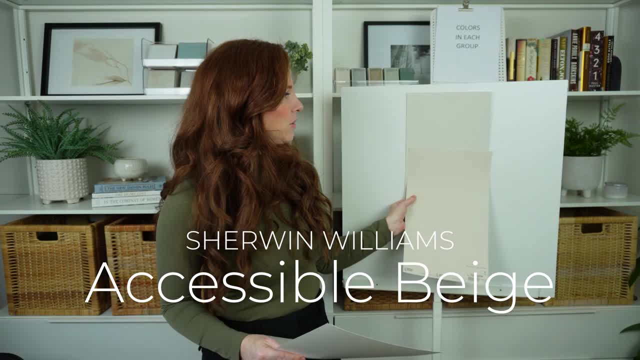 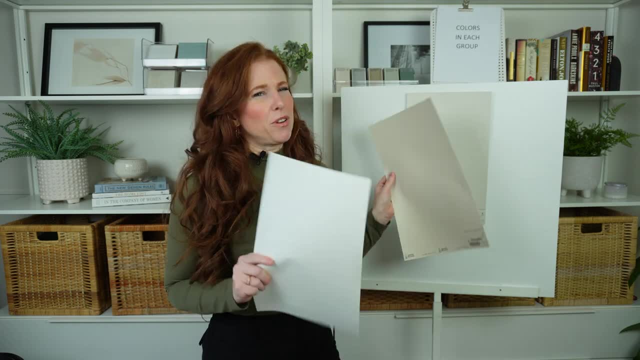 these colors. Now, if your home suits, agreeable gray probably doesn't sit in. accessible beige: If it suits this, it doesn't suit that. they're doing different things. The funny thing is they both harbor a tiny, tiny negative green in them, which is really cool. But accessible beige I want to totally different. 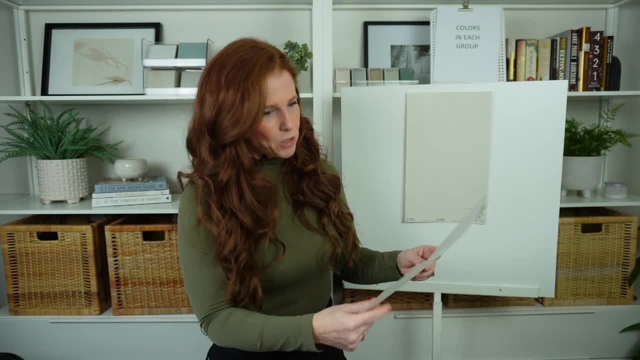 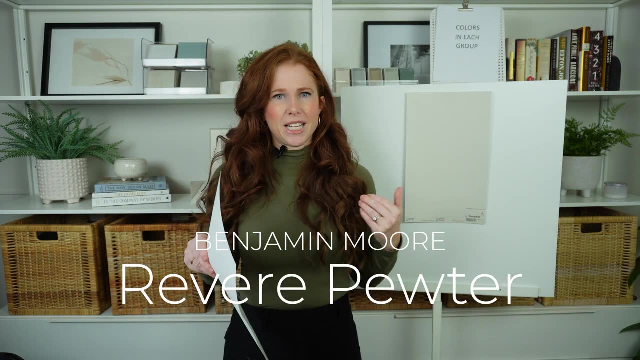 ballpark there and they're hardly comparable. Benjamin morelet's do. I don't want to do that one. Let's do Benjamin more Revere pewter. Now let's say you heard agreeable gray might be Earthy, warmясы, more muddy, a little bit of a green undertone. you look at it and go, oh, I'm kind of underwhelmed. I. 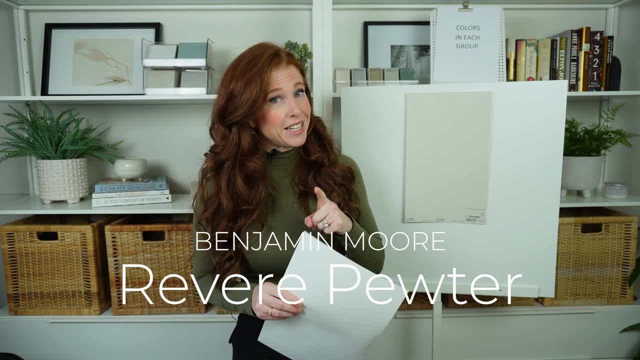 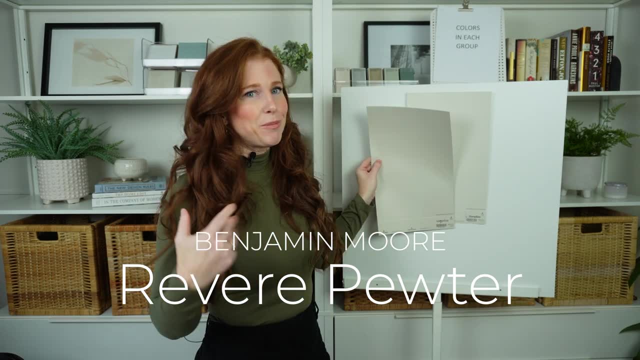 was looking for more well, you could look at Sherwin-Williams- amazing gray, which is amazing. or you can look at Benjamin Moore, Revere Pewter, which a little bit darker, a little bit more muddy, and of the two, is a little bit more inclined to grab green again. all these colors they can, and 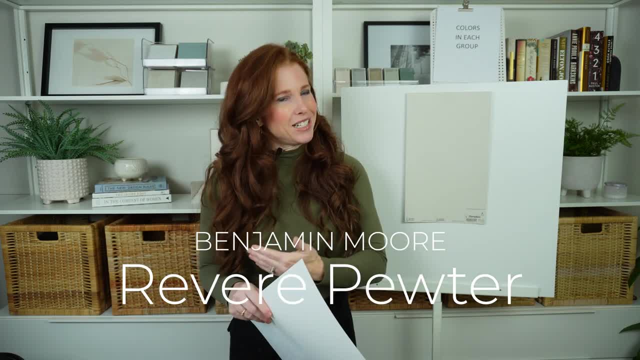 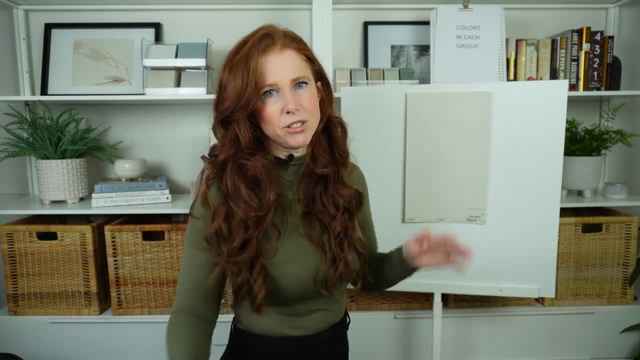 will change with exposures, lighting, all that stuff. this is just a place to start your sampling. you could check out the video on Revere Pewter and see more green options on that. so, and if they're not there, I'm doing a new video soon. hang tight. now we're going to look at white trim colors, so 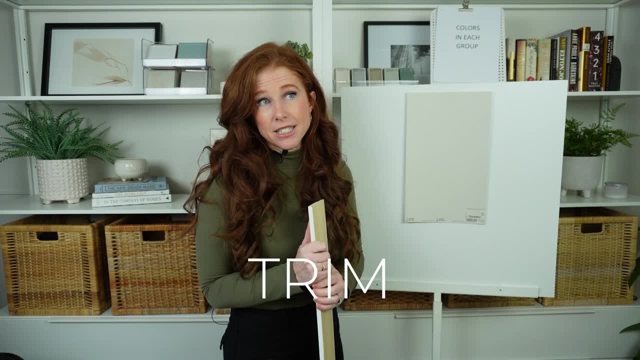 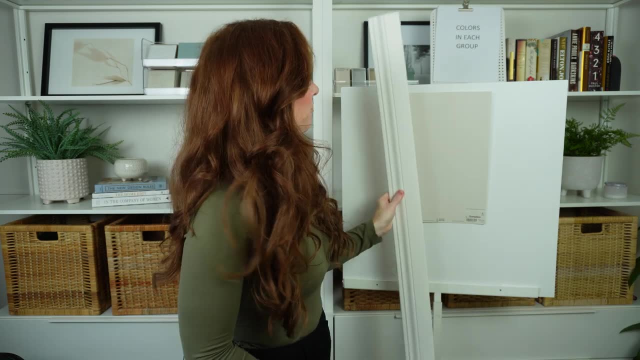 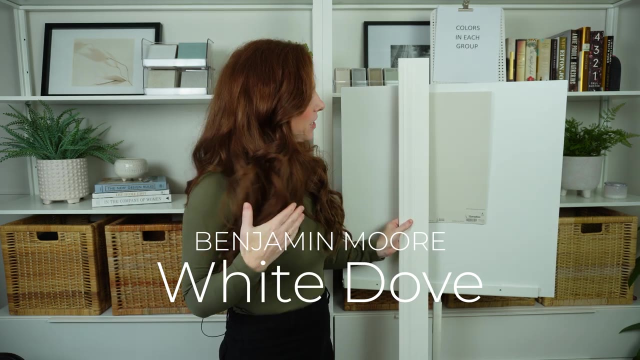 we can see which whites look best if you're looking for your cabinets, trim, ceilings, doors. now this fella here. I have to get these cut down, but it's on my to-do list. white dove- Benjamin Moore white dove looks gorgeous with agreeable gray. personally, this is about as warm as I'd like. 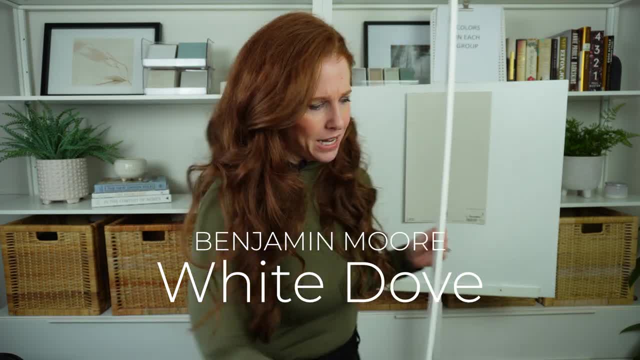 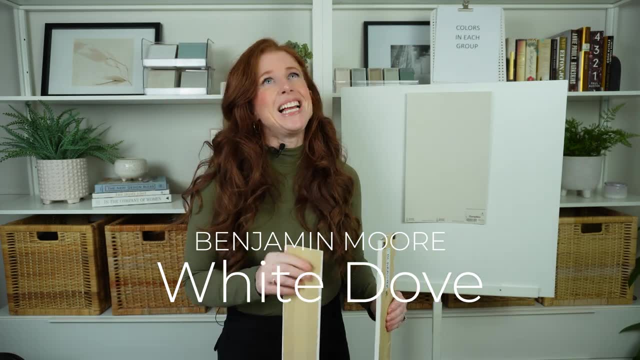 to go. let's look at Sherwin-Williams alabaster- where are you okay? so a lot of people like to partner agreeable gray with alabaster. it's doable. it's just if I could start from scratch, paint a room or a whole home from scratch. 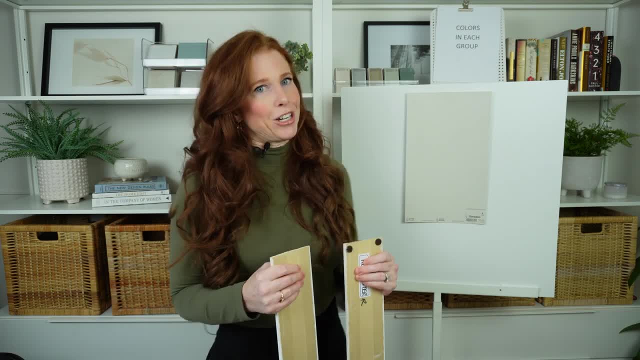 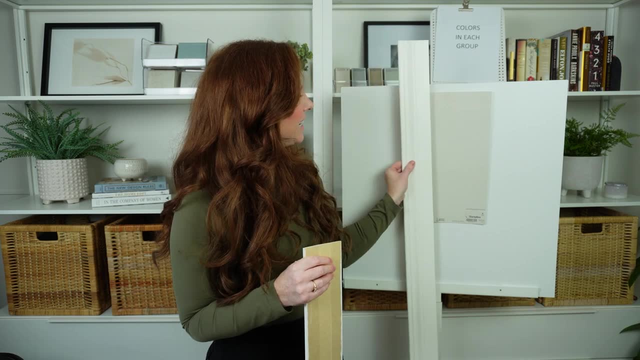 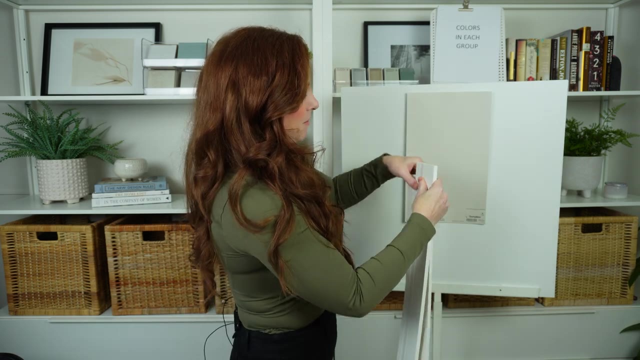 would I put agreeable gray and alabaster together? no, there's better options. so I would say it's doable. but you really want doable. you kind of want awesome. um, yeah, it's okay, you can tell I'm super excited about it. let's look at the difference here. sometimes it's comparing again. never just pick a color based on. 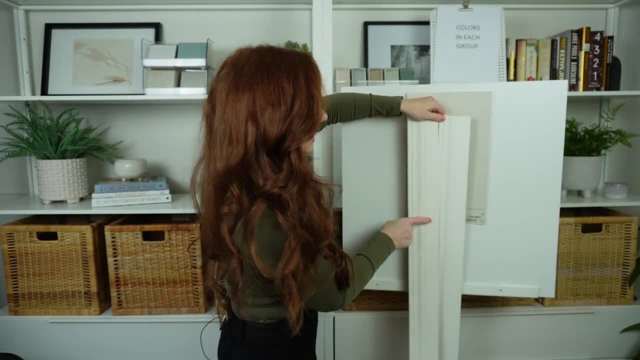 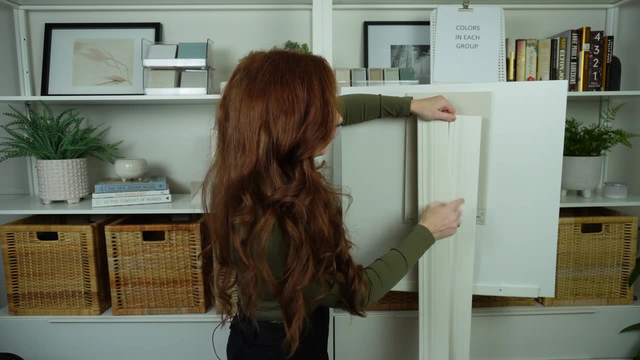 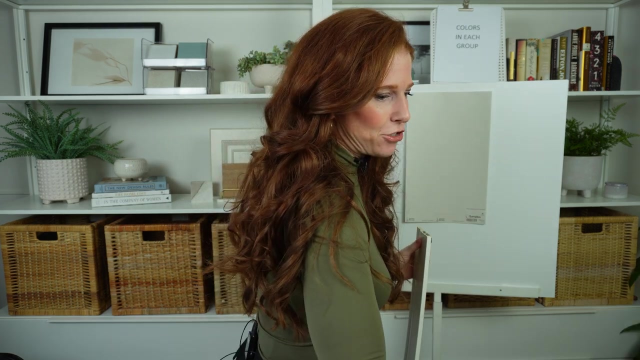 itself. so here's the difference: alabaster a little bit more of almost- I'll say slightly- dingy yellow, even though it's really pretty on cabinets. uh, white dove a little bit brighter. white dove's a way better choice if you have alabaster trim and you really want to use. 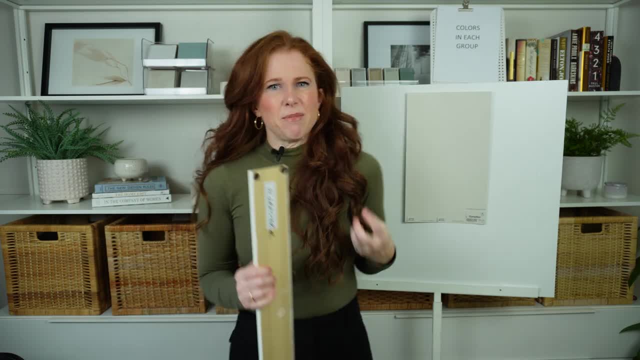 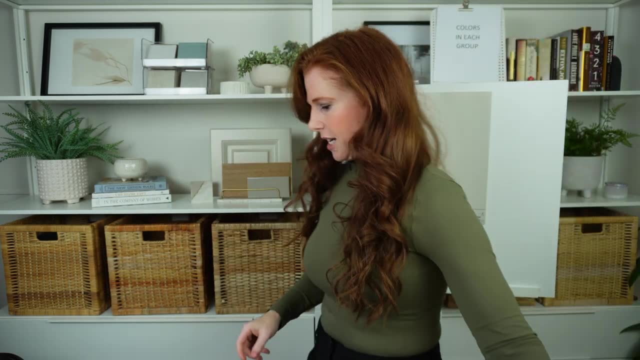 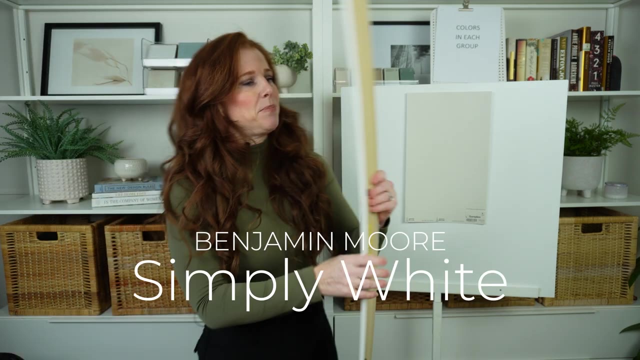 agreeable gray, maybe dark, and agreeable gray by 25. put a little more meat on its bones and it looks a little bit like alabaster, that little bit more. now you get to go away and we get to look at, not you. I don't want you to go away. talking to my trims, benjamin moore: simply white, this is a brighter. 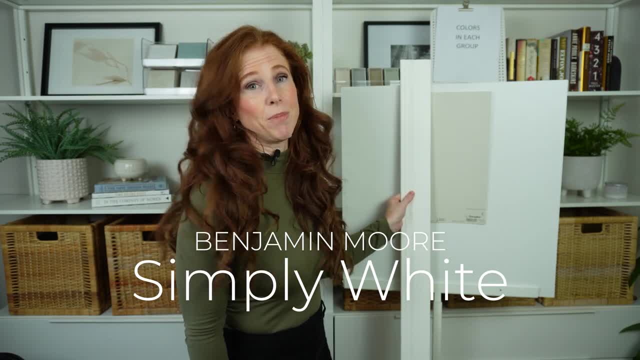 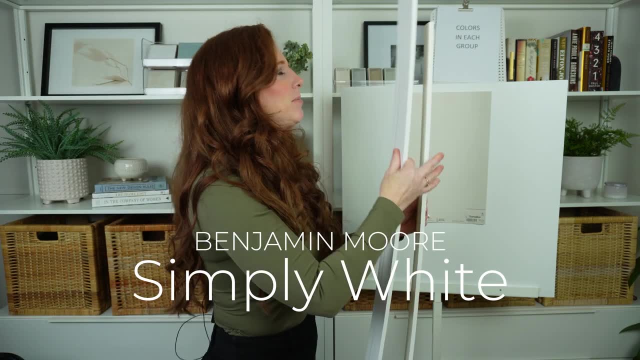 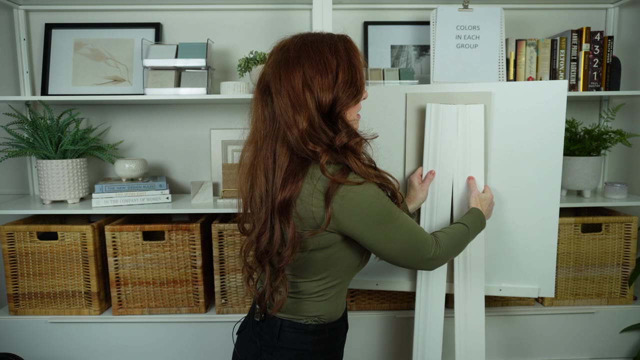 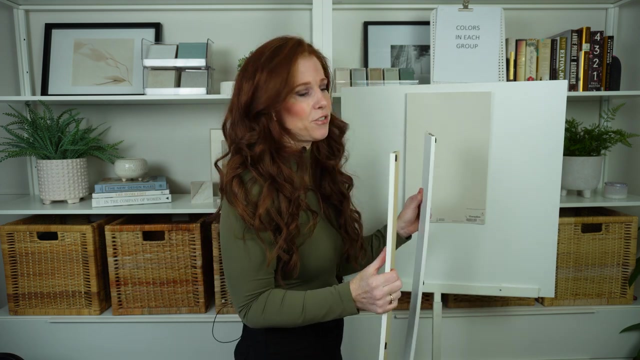 white with a bit of yellow. that looks great with agreeable gray. I have no problem with that. however, if I were choosing and starting from scratch, I would probably choose benjamin moore chantilly lace. it's a brighter white. there's your difference. that shift: a little bit more yellow here, a little bit brighter. chantilly lace is actually a slightly 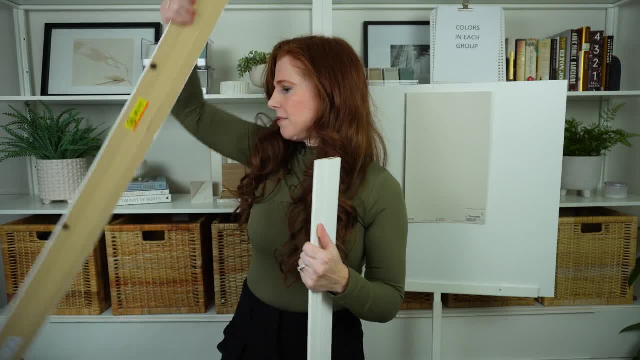 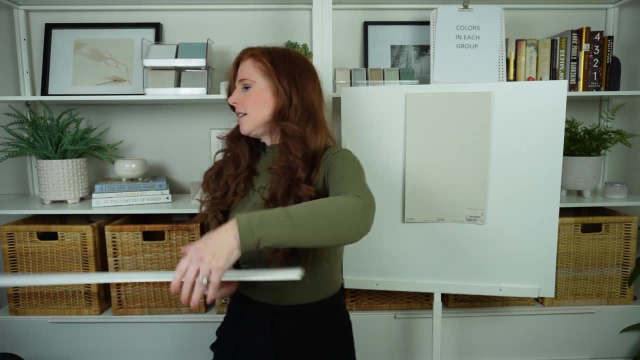 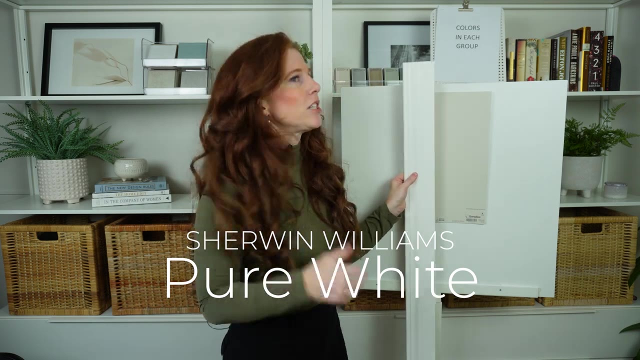 soft white, but you'd hardly know it. I like it with agreeable gray. but we're going to look at my numero uno twice. Sherman Williams, pure white, oh so pretty. eh, I love it. um, it's the perfect contrast. pure white has that super subdued, calm warmth. again, I have videos on all these. 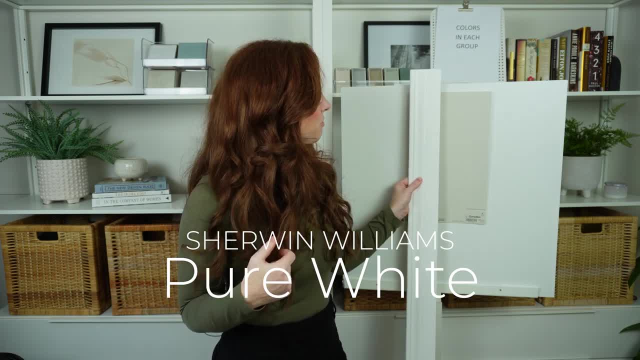 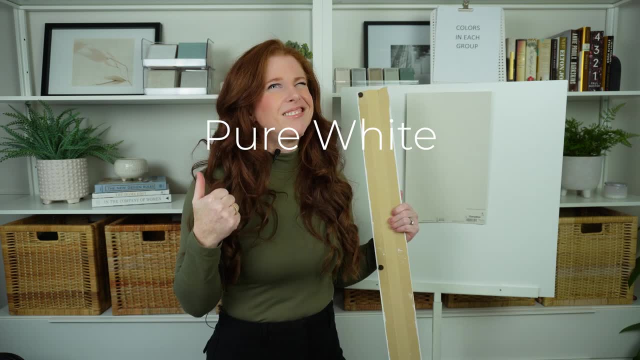 videos. I blog posts if you want to see photos of them. but if I'm starting from scratch and I have a choice- 100 percent pure white, pure white- then I'm going probably um chantilly lace or white doves, simply white alabaster is one of my last choices. but let me show you my very last choice. 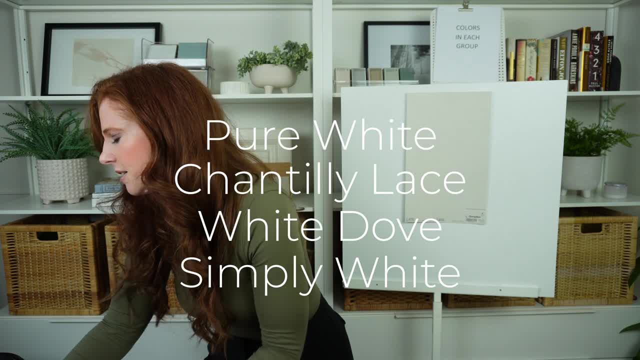 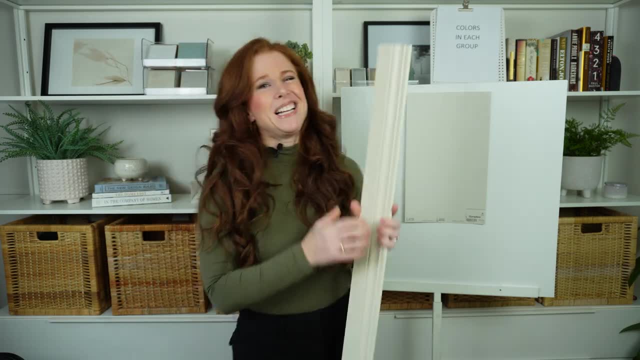 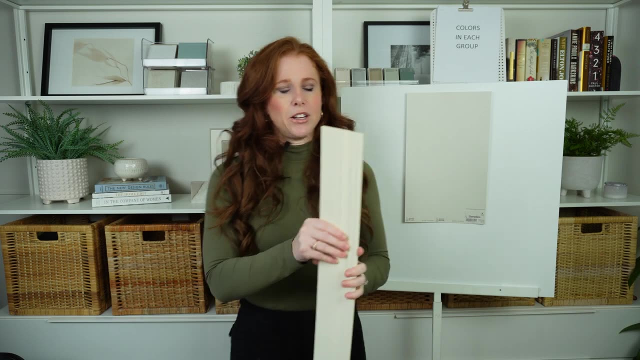 because some of you might be here because of it. oh, there's another one, Scherwin Williams, extra white. it's banging with agreeable gray. I love it. yeah. so some of you have cream trim or you're like, oh please can I put agreeable gray on my walls? it's the hardest dough I could ever give. 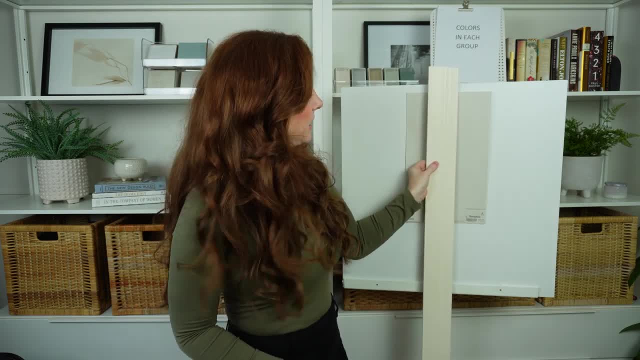 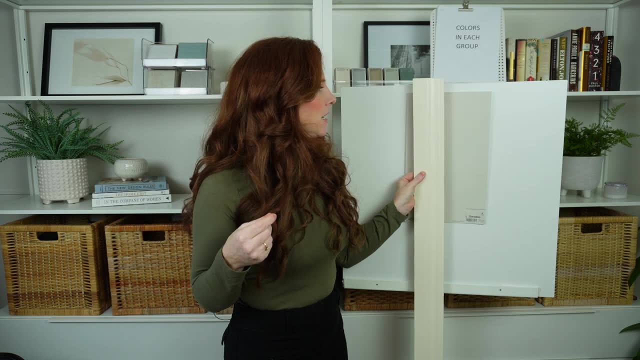 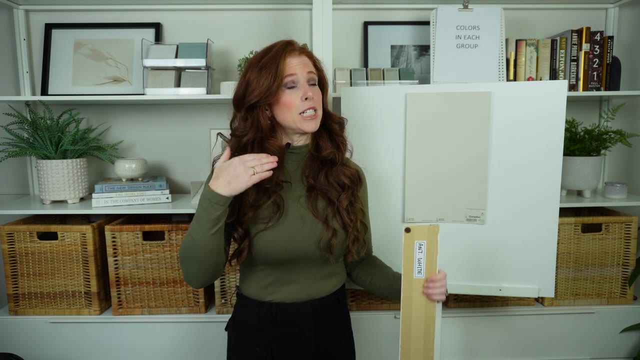 you right. I mean, if you look at that and you're like you know what, I'm okay with it. that's cool beans with me, but personally it's. it's not a great combo. I think I have a really long video on cream cabinets and trim. I know I have several blog posts. if you go into my search, I have blog.